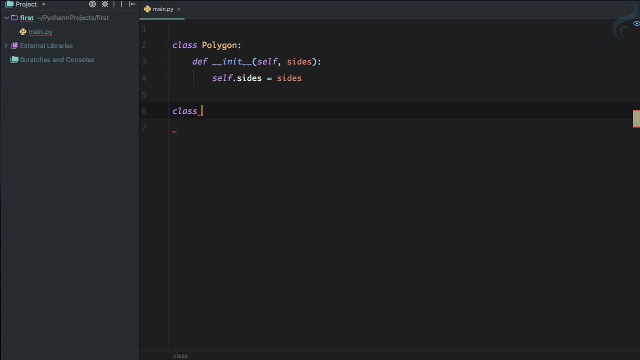 the sites given. so let's create another class and this class is actually a square. okay, so what we we want to do, we need to do same thing here, so and let's try to use the square method. so I will say square, sqr is a square, and now I will provide four, because this is on init method. so as we define the 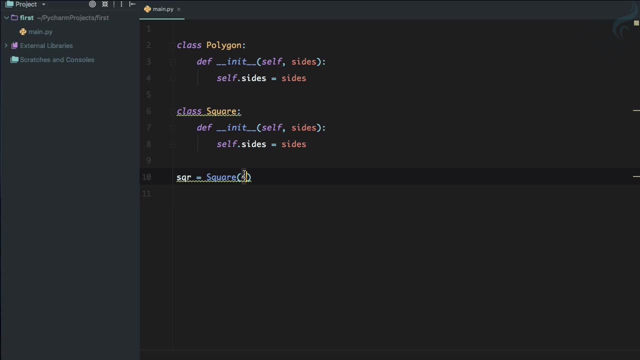 object or, as we initializing it, we need to give the sites. so this is good. and now if I say print a square, that means SQR dot sites, it will result to four. this is good, but you can see we are repeating ourselves. we are using the same thing in two classes, but you can see this square is. 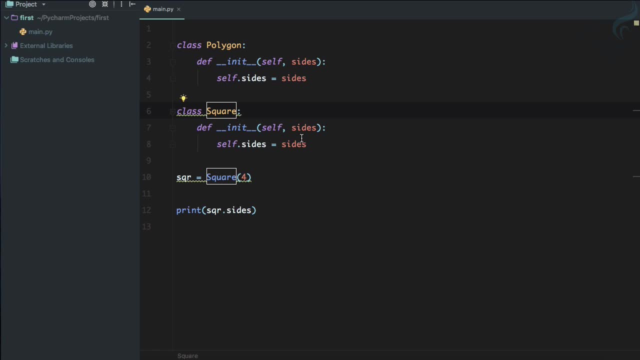 a polygon, so why not inherit this class? so how I can inherit the polygon class in Square class? it's very easy. you just need to use this parenthesis and in the parent synthesis let's define your class, which is polygon. so, because this is an empty class, if I try to run 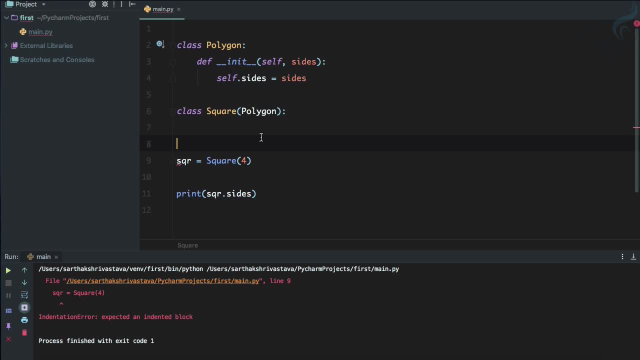 this. we are getting error because this class is empty and if a class is empty, you need to give a pass keyword so that python will go inside and it will say, okay, I don't have to do anything here, and because this is inheriting. so now, if I run it, yes, you can see we are getting full. but how this is? 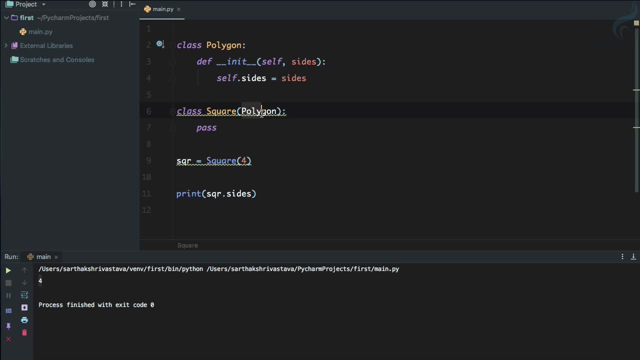 going to work. so let's see, whenever we are inheriting the any class with the bigger class or the parent class, then all the functionality of the parent class comes inside the child class. so here the parent class functionality. this init method is coming here, great. so we have used that sites functionality just by using the square class. so let's create another. 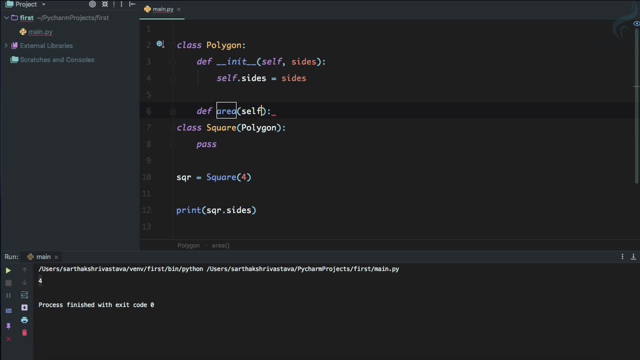 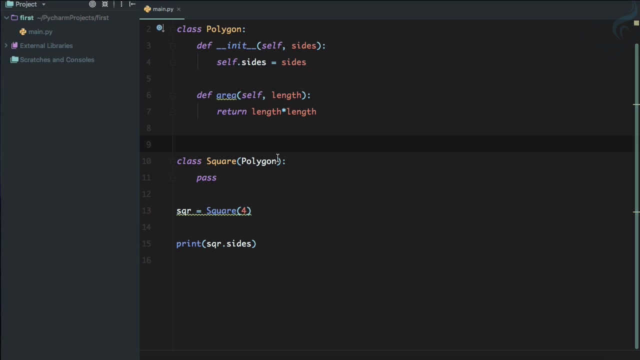 function here and this function is called area and you know, square uses just the length to find the area, so it just return length. uh, you just return length, multiply by length. that's it. so how we can do this things now, because we are again inheriting, we can use the area function of this polygon class from 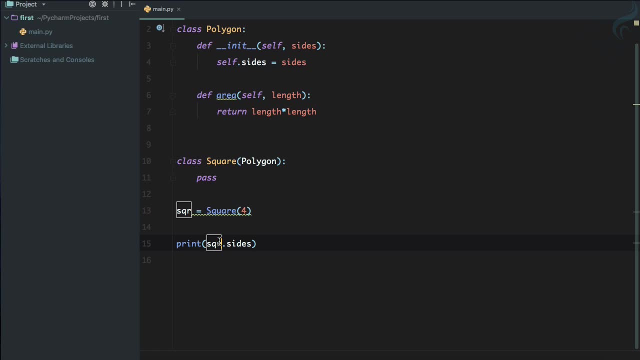 our square object, so square dot area with, let's say, I will give 5 centimeter. so if I run it 5, 5, the 25 is here. so we are getting the answer. so this is because of the inheritance, but suppose I create another class, so class of. 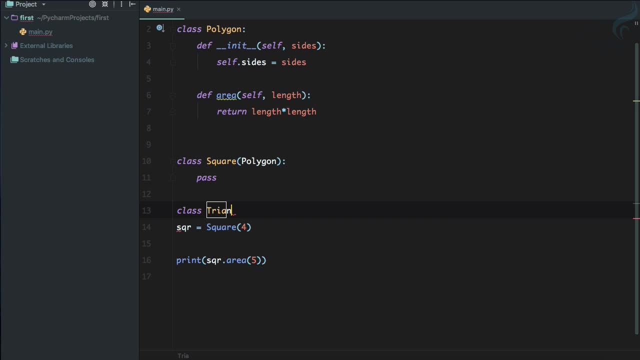 say triangle, so triangle class I have used and it's also a polygon, so I can inherit polygon class inside this triangle class. that's good and we need to give the pass statement. but you can see these two things. that means square and triangle doesn't have the same formula for creating the area, so one. 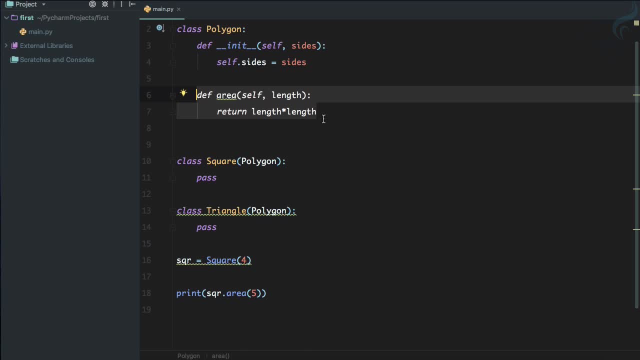 thing, what we can do, because we don't want to use this formula. we want to create a new formula for triangle. we can rewrite that function. so the same function I'm writing here. but this time, if we try to use this function, it will call from triangle method, not from the polygon. so let's first complete this, so it will. 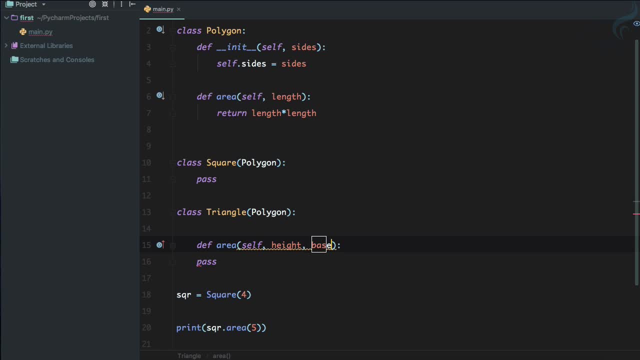 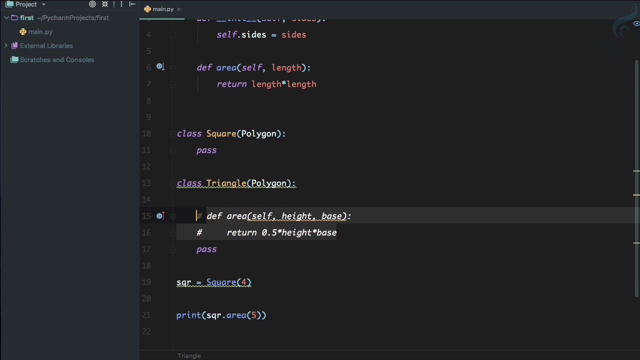 say height and base. so now it will be like returning of 0.5, multiply by height, multiply by base. this is the formula for using the area, calculating the area of a triangle. okay, so now what I am going to do. let's just comment this out for now. create a. 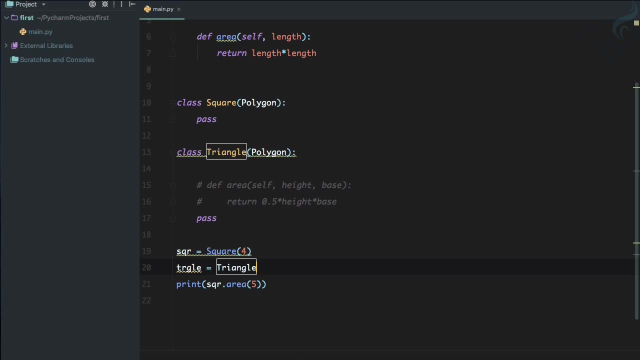 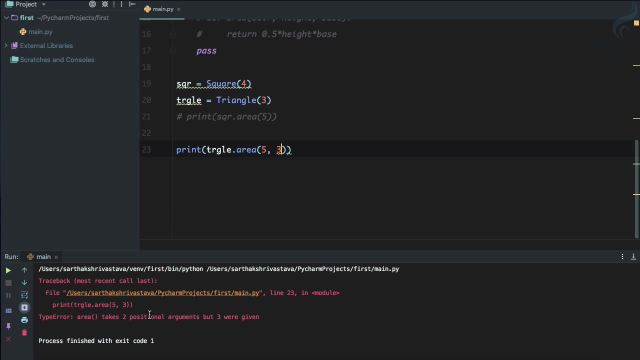 new object of triangle class, providing the sites, which are three, and this time I'm going to print triangle dot area and let's give two things: one is height and another is, we know, base. but if we run this we will get error because this is saying that area take two position argument, but three. 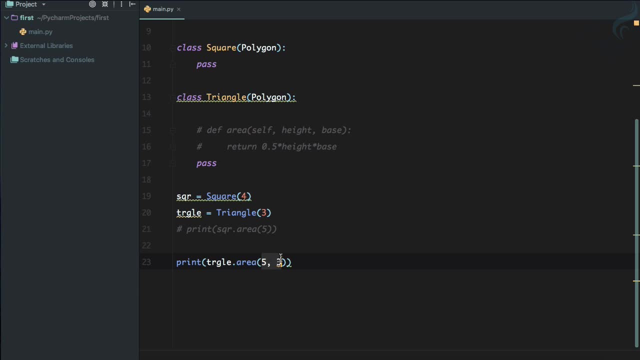 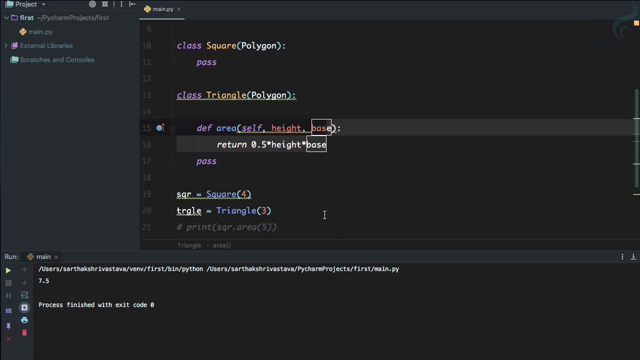 given obviously three, because two are argument and one is actual self. so it required two. we have given three total. so this is giving error. but what if I uncomment this and try to run again? and yes, you can see we are getting the area, which is 7.5. why this happens? because we have overridden the area function, or 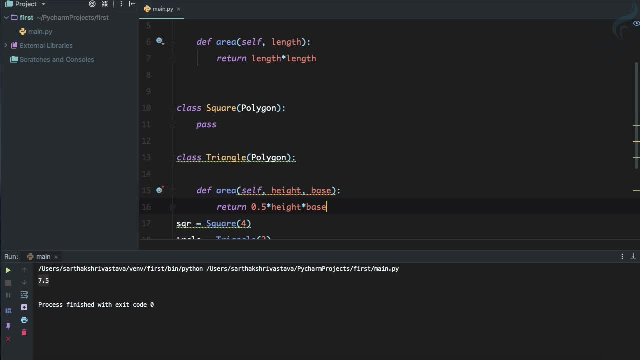 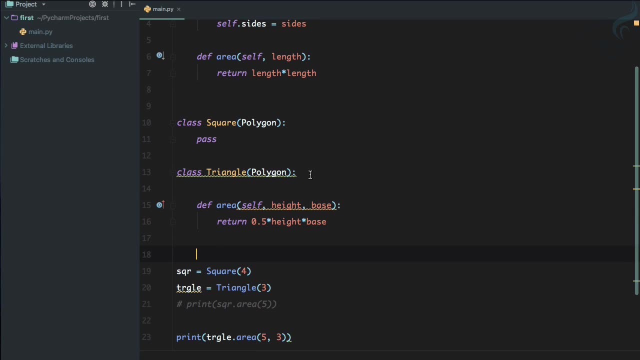 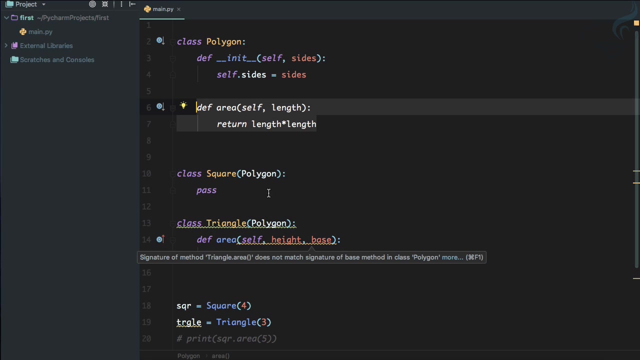 area method from here. so now we can just remove the pass method and still it's going to work fine. so this is very, very useful thing in inheritance that you can overwrite any functionality you want. so this is very nice. you can see this square class is looking empty, but because it is inheriting, it has these: 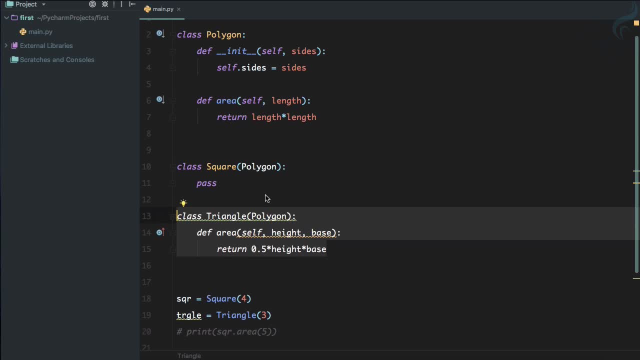 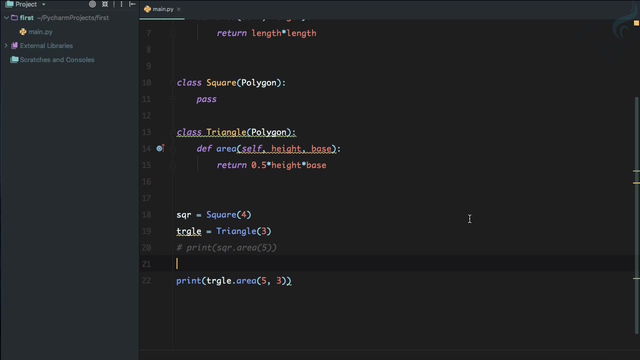 two functions. and again, this triangle class also has these two functions, but this one, the area function, we have overridden. let's just use some of the built-in functionality to check who is the instance of which class. so I'm going to print and I will say: is instance. so I'm going to check if square sqr is an instance of a square or not. so 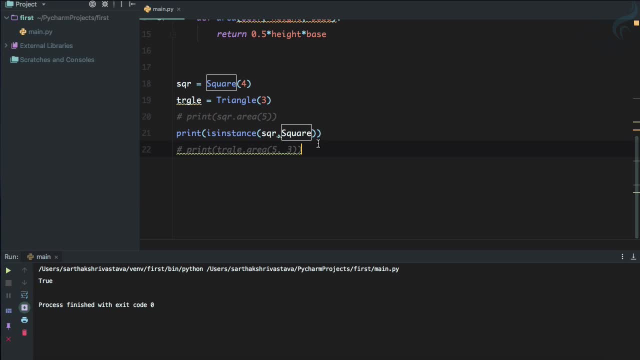 let's just comment these things and try to run it, and it says, yes, sqr is an instance of a square. but what if I say triangle? try to run it. it says, no, this is not an instance of triangle. but what if I say polygon is interesting? and yes, it's saying true, it's not an instance of a square, no, it's an instance of a. 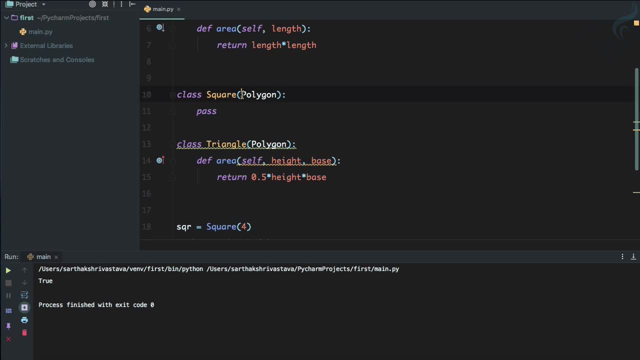 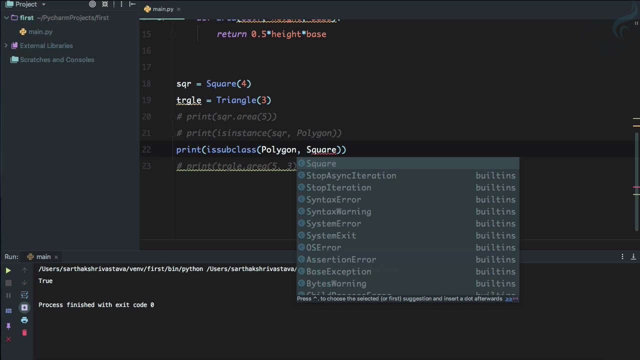 square, because actually the square class is also inheriting the polygon class. so, similar to is instance, there is another function which is called is subclass, so some class of any other class or not? so let's just check. so we need to check this. so obviously this has to be with capital P and capital S. run it and it says: 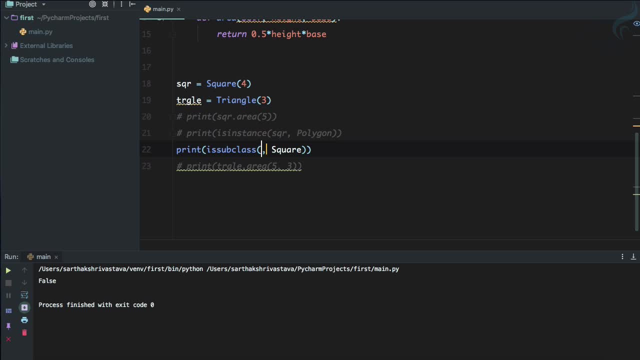 no, this is not a case. so what if I change the positions- and we know this is going to be true- and run it? and yes, it is true. so this means we can check whether any class is an instance of other class or not. these things are good, but what? 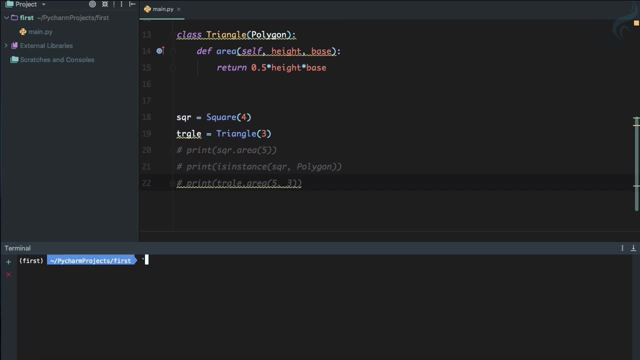 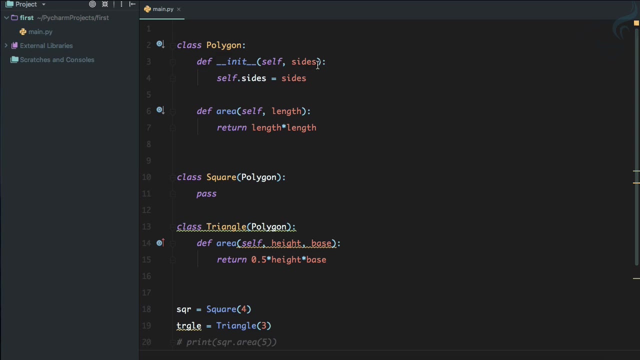 if you want to add some functionality to your class, but that functionality is not available in the polygon class. that means the base class. so here you can see, we have the sides. but what if I try to define the init method here, and here I will say not side, I will say square. 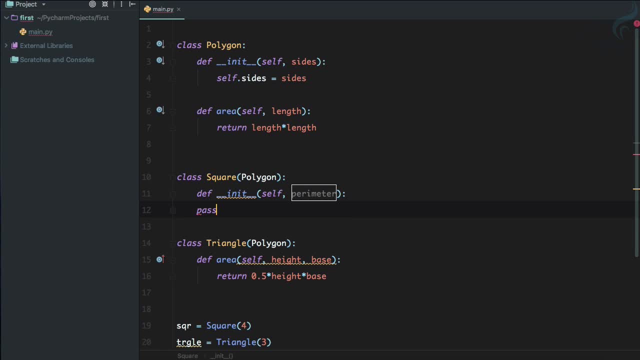 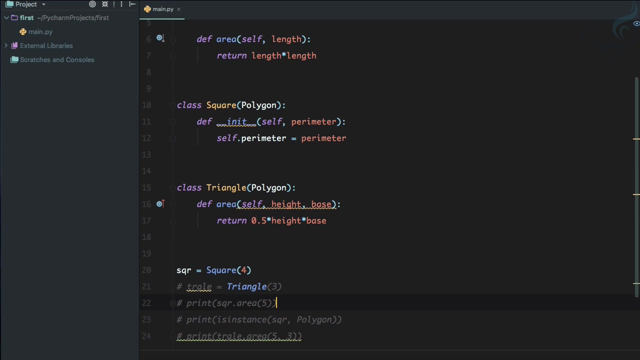 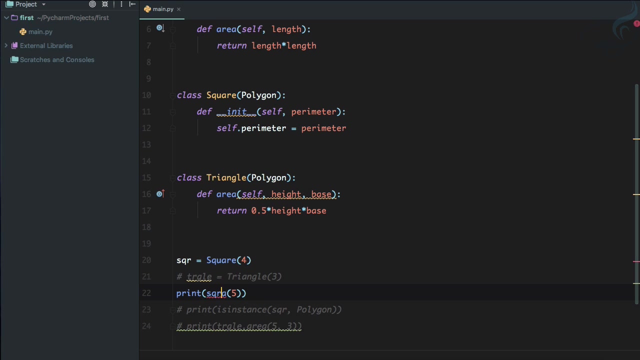 parameter. so I'm going to get the parameter and not any pass. so I will say: self dot: perimeter. perimeter is equal to perimeter. okay, so we have done this. so what happened to this system? if we try to use a square instance and getting the parameter of a square, so let's try to use the. 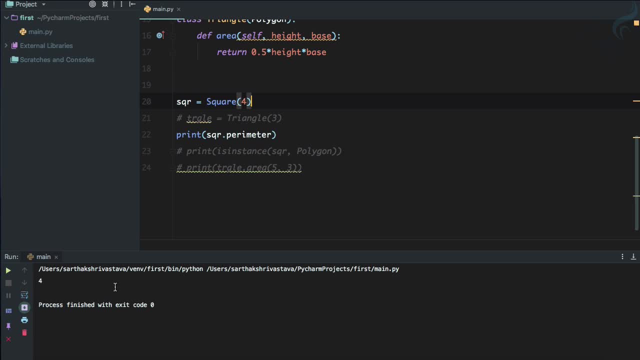 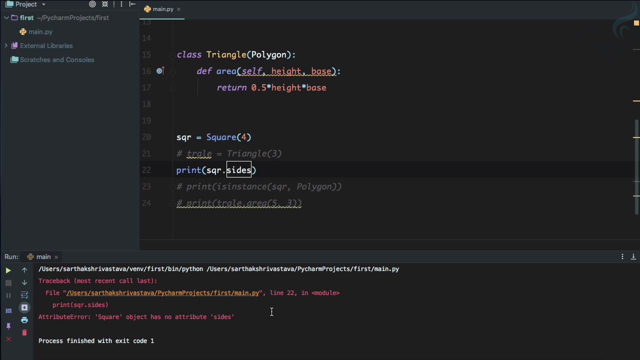 parameter. and let's see it's saying four, but we want the side also, the sides also and the parameter also. so how we can get that? so let's try to get the sides. okay, it says error. it says there is no attribute called sites. why this happens? because you know, this init method is overridden by this init method of polygon.